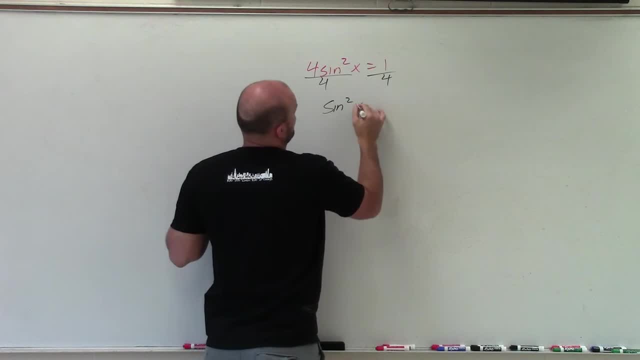 to divide by 4 on both sides And I have sine square root of x equals 1. fourth, Now I need to undo the square root, so I'll take the square root of both sides. So if I have sine of x equals, now remember, the square root of any rational term can be written as the: 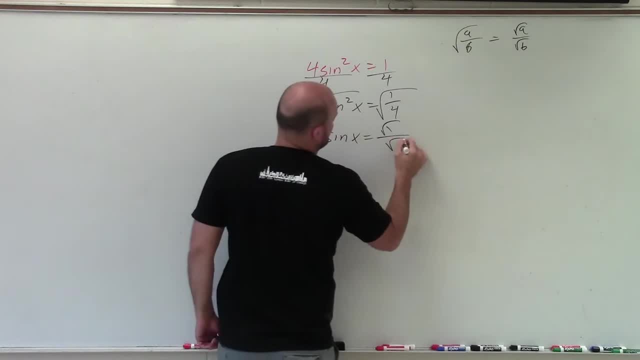 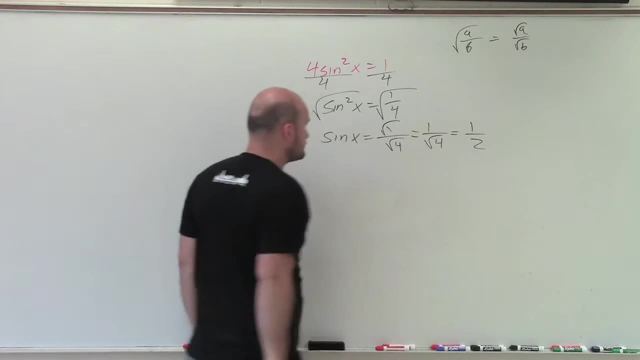 square root of a over the square root of b. So this is equal to the square root of 1 over the square root of 4.. Square root of 1 is just 1.. Square root of 4 is equal to 2.. So 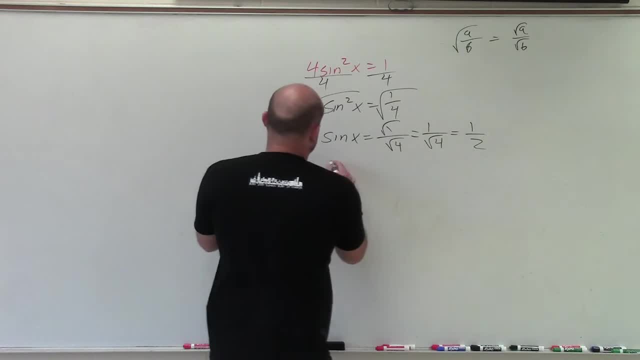 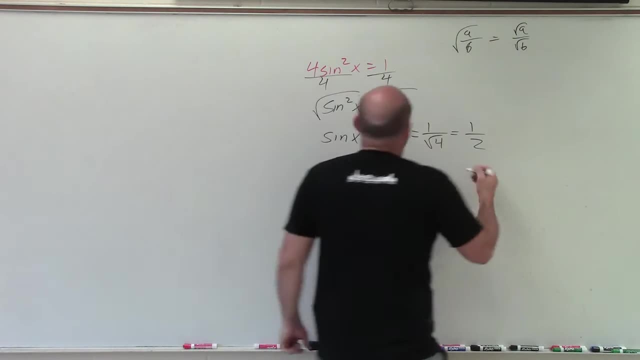 I have, the sine of x is equal to 1 half. So now to determine our solutions of for what angle is the sine of whatever that angle we're looking for, equal to 1 half? So to do that, we go to our left. 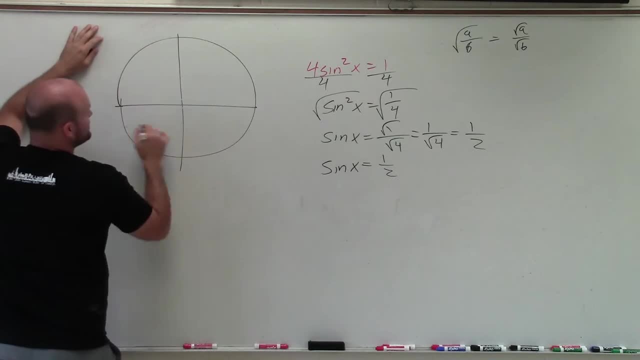 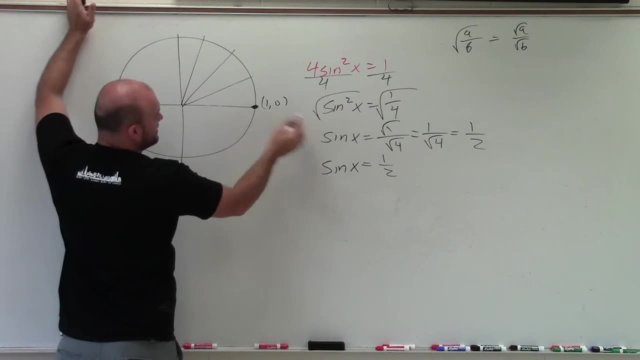 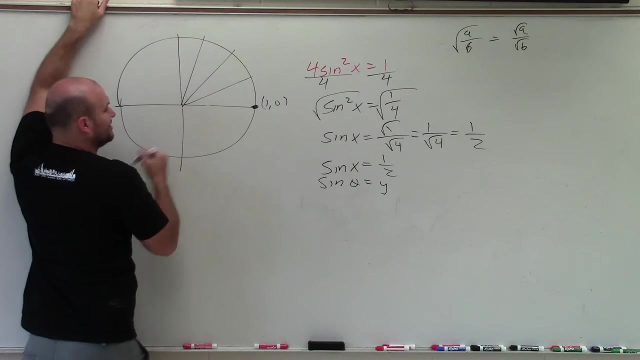 We have our lovely unit circle And we just go ahead and look at the first quadrant. Our first point at 0 is the point 1 comma 0.. Well, obviously the number sine of any angle is equal to the y coordinate of your point on the unit circle. So obviously my y coordinate. 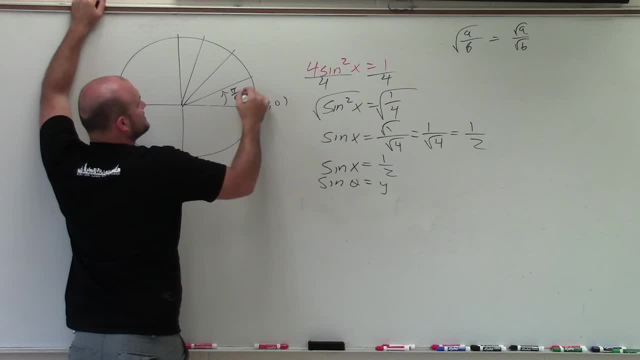 is not 1 half there. Let's go to the next angle: pi over 6.. Well, that angle is square root of 3 over 2 comma 1 half xy. Guess what? Ding, ding, ding, ding ding. We found our. 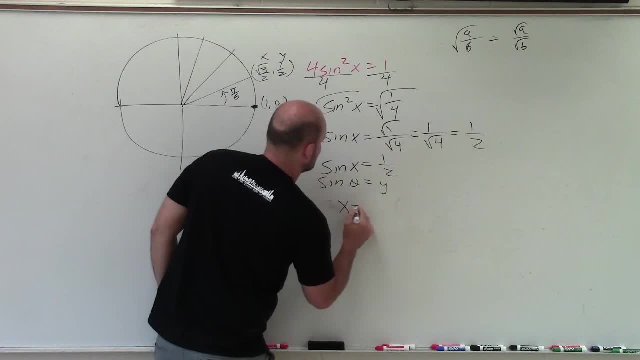 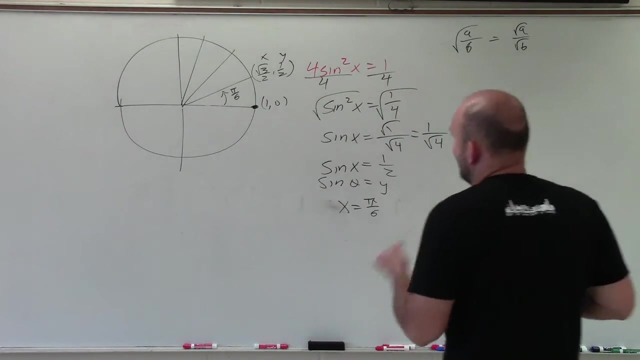 first answer. So therefore I can say x is equal to 1 half, Meaning that x is equal to the angle pi over 6.. But that's not the only angle that x is going to equal to 1 half in this first quadrant. 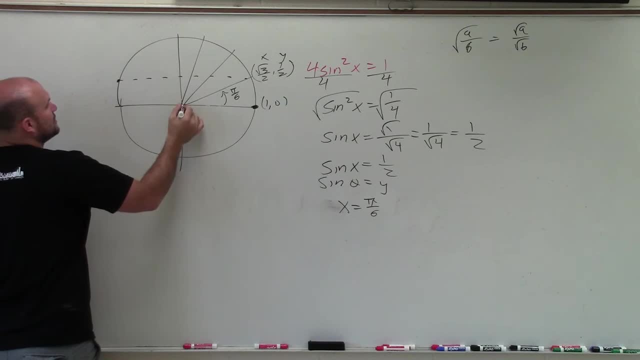 It's also going to equal to 1 half, with the reflection over in the second quadrant. That angle Why? Because this angle, which is 5 pi over 6, has a reflection over here And has a point of negative square root of 3 over 2 comma. 1 half xy. 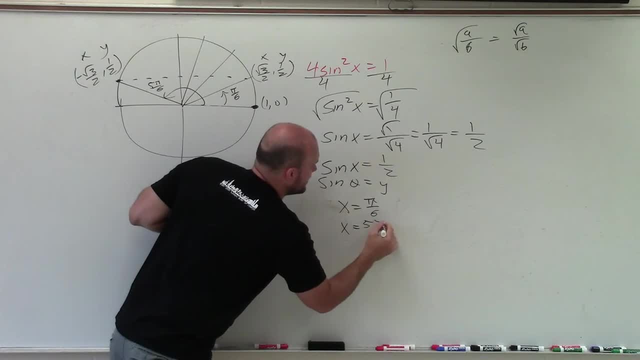 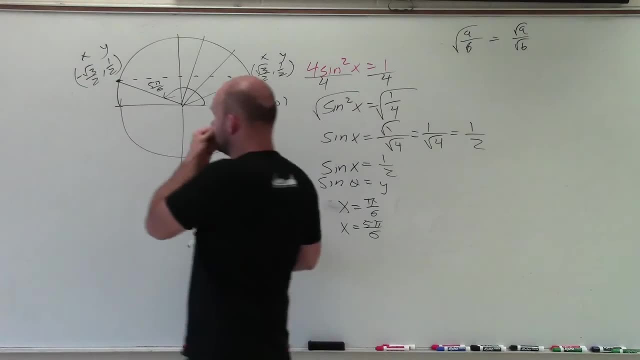 So now we have actually two solutions between 0 and 2 pi. However, what we're trying to do is determine all of the solutions, So therefore, I need to determine: well, how am I going to determine all my solutions Now? remember when we found coterminal angles. 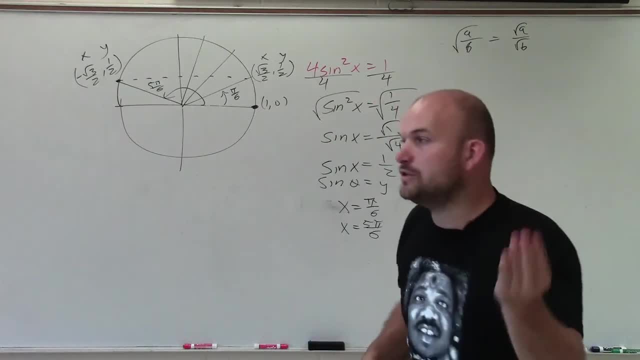 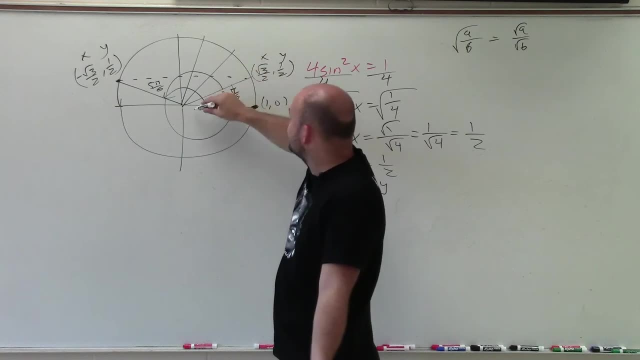 coterminal angles allow us to determine multiple revolutions just by adding 2 pi. So if you're about pi over 6, if I add 2 pi over here, I'm going to get back to that same angle And so it's going to be another solution.